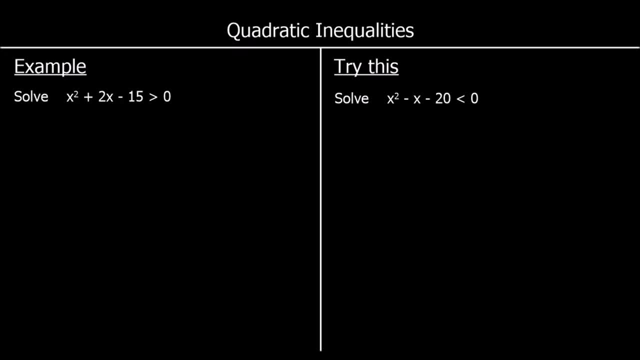 This question says: solve x squared plus 2x minus 15 is greater than 0. That means we're looking for the values of x that make x squared plus 2x minus 15 more than 0. It's easiest to explain what we're looking for by looking at the graph. 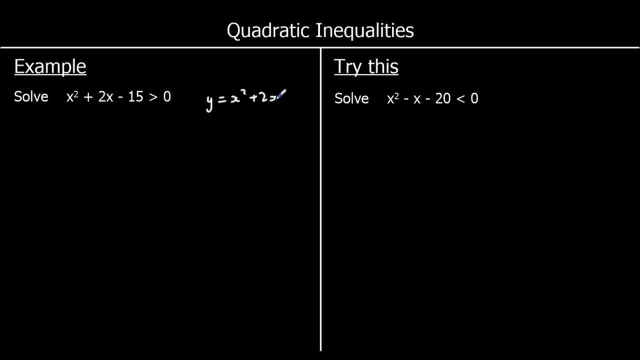 So let's look at the graph of y equals x squared plus 2x minus 15.. And that will look something like this: So it's a positive x squared graph, It's a positive u-shaped graph, And if we find where x squared plus 2x minus 15 is equal to 0,, 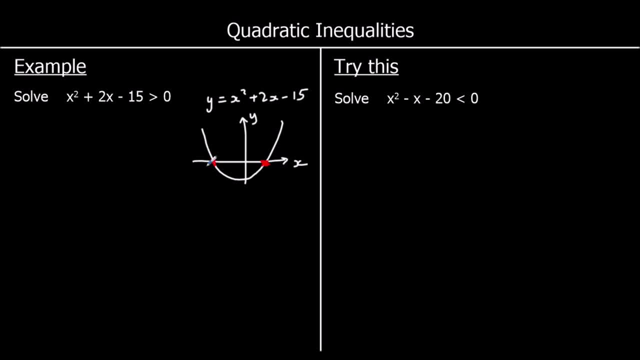 that will be the two points where it crosses the x-axis. So if we find where it's equal to 0, that's the points where it crosses the x-axis. So if we find where it's equal to 0, that's the points where it crosses the x-axis. 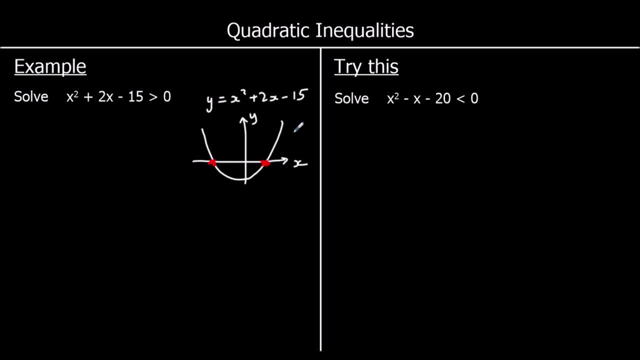 And it's greater than 0 above the x-axis. So we're looking for these two parts of the graph here. So we're looking for what values of x, what the values of x are for these two parts of the graph. So let's find out where it crosses the x-axis first. 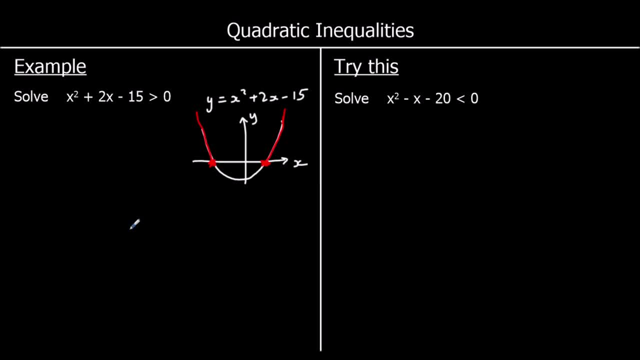 And we do that by solving a quadratic, like we would usually. So we can solve this by factorizing. So we're going to have double brackets, We're going to have x in both brackets. x times x makes x squared, And we're going to look at what numbers multiply to make negative 15. 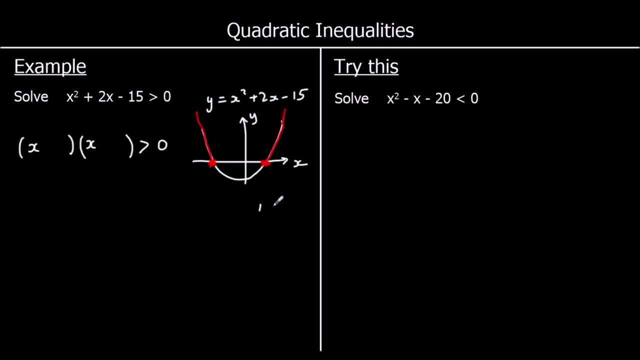 and add to make a positive 2.. So we can have 1 and 15 or 3 and 5. They are the numbers that multiply to make 15.. How can I make a positive 2?? That's with 3 and 5.. 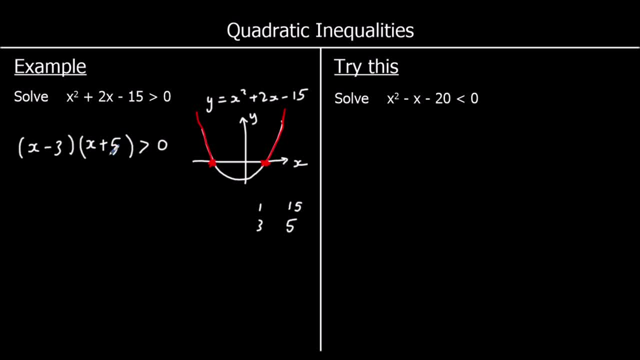 And it's negative 3 and positive 5.. So what are the x values here where it crosses the x-axis? So it crosses x-axis at x. What makes this first bracket 0?? That's when x, That's when x. 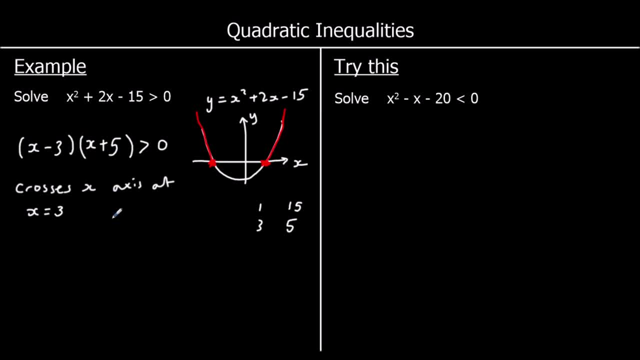 x is 3.. 3 minus 3 is 0.. And what makes the second bracket 0?? That's negative 5.. So this is negative 5 and positive 3.. So what is the answer? So this red bit of the graph on the left is where x is less than negative 5.. 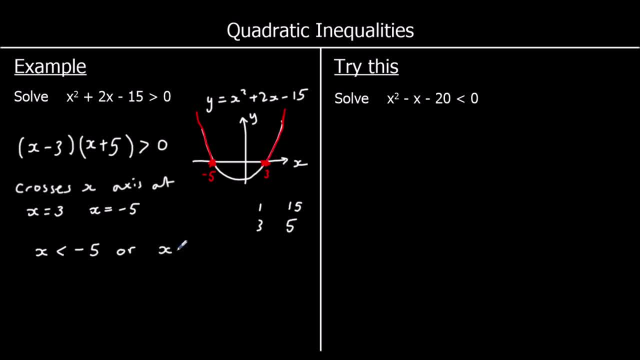 And the bit on the right is where x is less than negative 5.. And the bit on the left is where x is less than negative 5.. And the bit on the right is where x is bigger than 3.. are anything bigger than 3.? 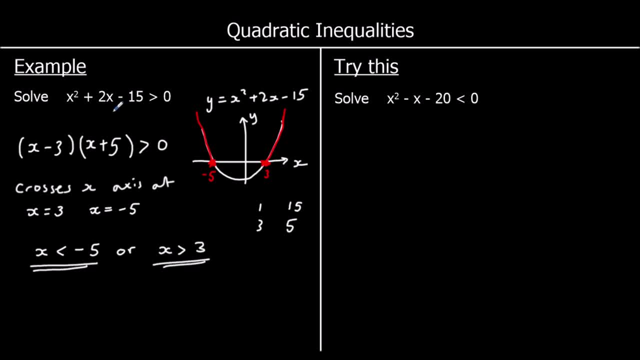 We'll make this x squared plus 2x minus 15, bigger than 0.. Okay, one for you to try. So if you feel ready to have a go, give it a go. Otherwise just keep watching. So the difference this time is it's less than zero. 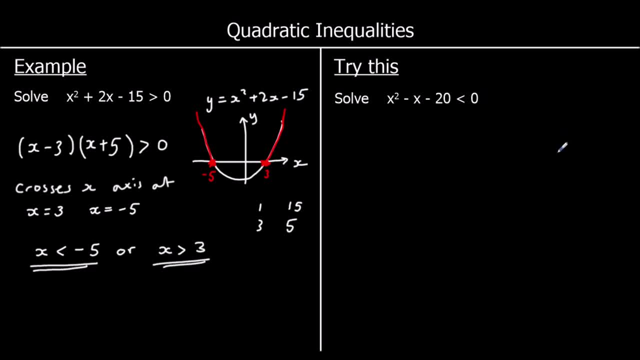 So that's a key difference in this question. So, if we look at the graph of y equals x squared minus x minus 20.. Again, it's a positive x squared graph. So it looks something like this, And this time we want to know where it's less than zero. 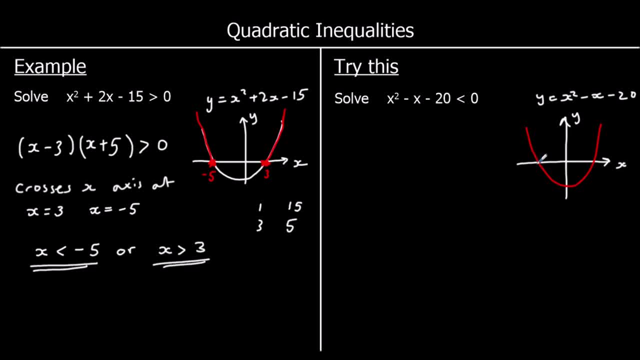 So where is this graph? less than zero, Remember. it's equal to zero when it crosses the x-axis. It's less than zero when it's below the x-axis. So we want the values of x for this part of the graph. So, again, we're going to find the points where it crosses the x-axis first. 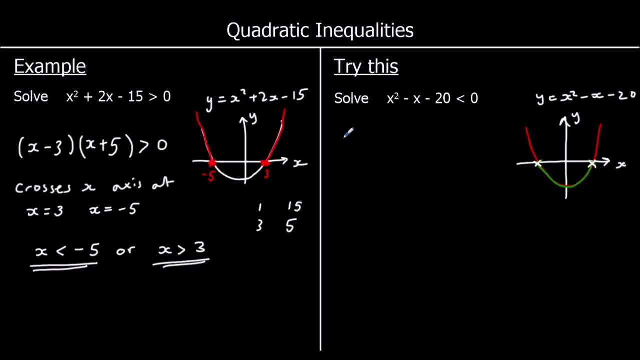 So we'll solve as we normally would, by factorizing. So we're going to have double brackets x. in both brackets What multiplies to make 20? 120,, two 10s or four 5s? Which of those can give me a negative 1?? 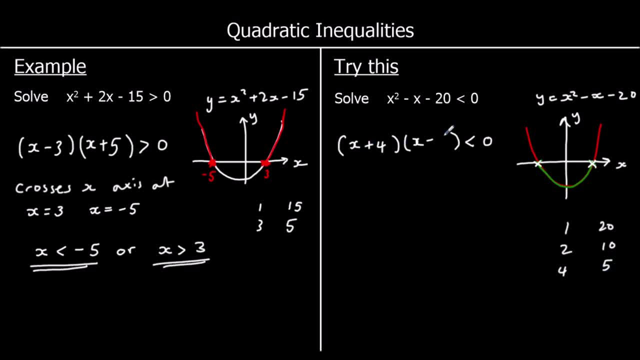 It's 4 and 5.. So I'm going to have plus 4 and minus 5.. So where does it cross x? So it crosses x At what makes the first bracket zero, That's negative 4.. And what makes the second bracket zero? 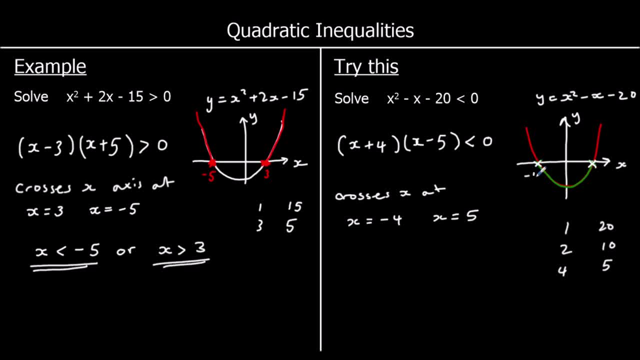 Positive 5.. Negative 4 and positive 5.. And we're looking for the bit of the graph below the x's. So what are the x values in this part of the graph? Well, it's in between Negative 4 and 5.. 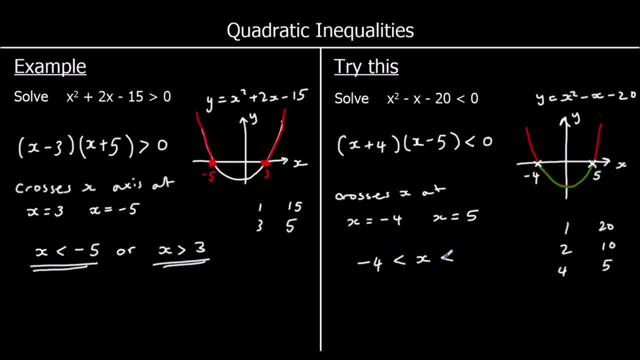 So we can say that x is bigger than negative 4, but less than 5.. So in between negative 4 and 5.. So anything between negative 4 and 5 will make this x squared minus x minus 20, less than 0.. 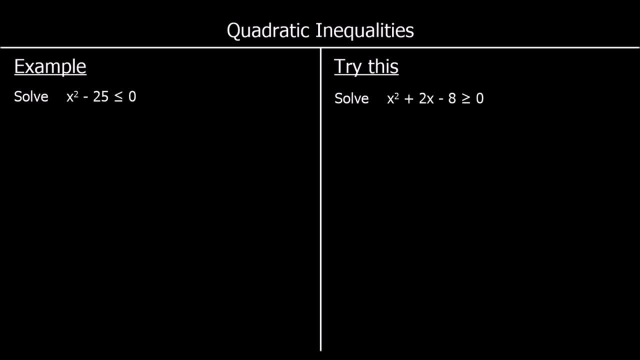 And another example Here. this time, instead of the symbols being less than or greater than, we've got less than or equal to and greater than or equal to. But otherwise it's the same sort of question. The first example: x squared minus 25 is less than or equal to 0.. 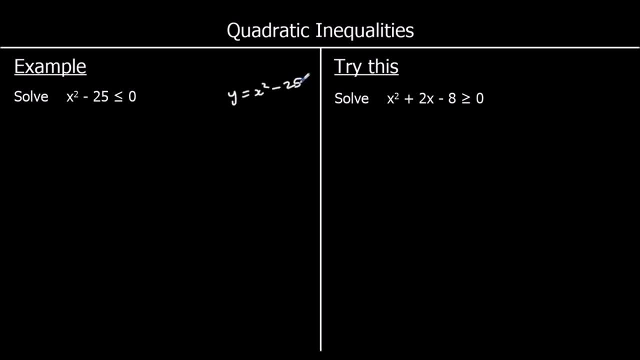 So let's quickly sketch x squared minus 25.. So the graph looks something like this, And we're going to do the same thing: We're going to find the two points where it crosses the x-axis, We're going to find what makes it equal to 0.. 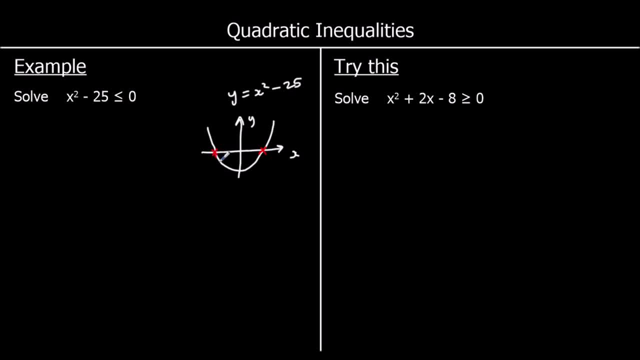 And we want less than that's under the graph, And then, once we've found those two points, we can write down What would make it less than or equal to 0.. So we're finding the lower part of the graph, the bit underneath the x-axis. 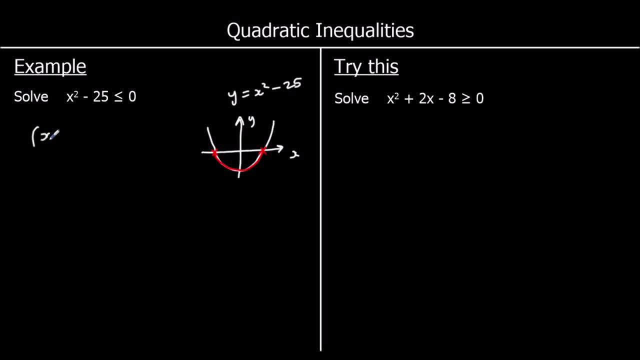 So let's find these points. We do that by solving normally And we're going to factorize. And x squared minus 25 is the difference of two squares, So it's x plus 5 and x minus 5. 5.. 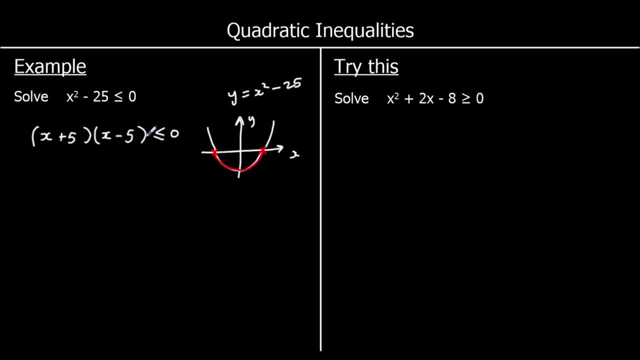 5 and negative 5 multiply to make negative 25.. And they add to make 0.. And we've got this. So now we can say that the points where it crosses the x-axis are x equals minus 5 and x equals plus 5.. 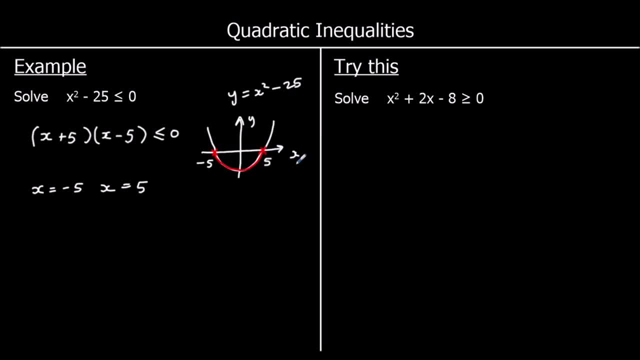 This is negative 5 and positive 5.. So what is the red bit of the graph? So it can be anything. It can be anything in between negative 5 and 5, but including negative 5 and 5 because it can equal them. 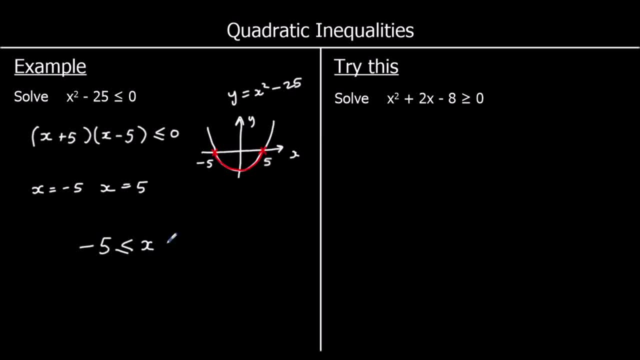 So it's: x is bigger or equal to negative 5 and less than or equal to positive 5.. Okay, one for you to try here, So give this one a go. Okay, So we've got solve: x squared plus 2x minus 8.. 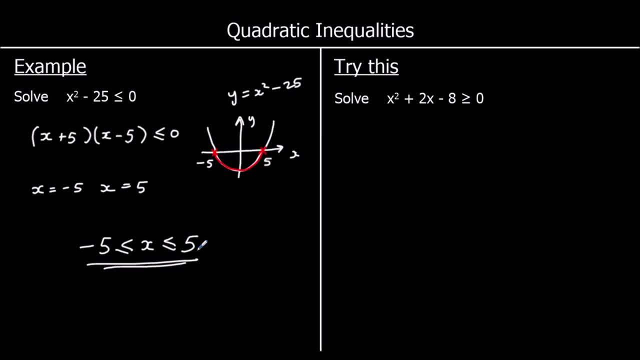 What does that write? Time is 0. So what does the break? j is equal to 0. And $0 is positive because it's given. So $0 is greater than or equal to 0.. So, again, if we look at the graph, we're going to have something shaped like this: 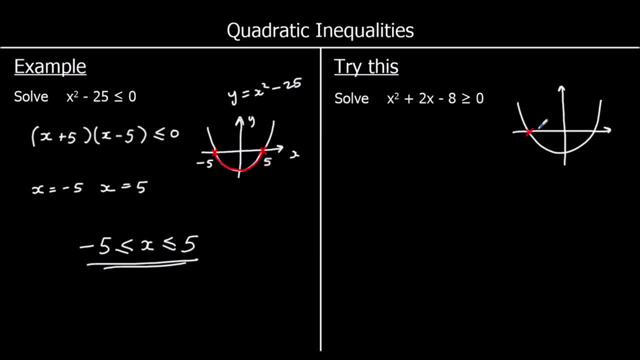 And we're looking for above 0.. So it's equal to 0 where it crosses the x-axis and it's bigger than 0 on these parts of the graph. So let's find out where it crosses the x-axis first. so let's do that by factorizing. so what multiplies to make 8 negative 8, we 1 and 8, or 2 and 4? how can? 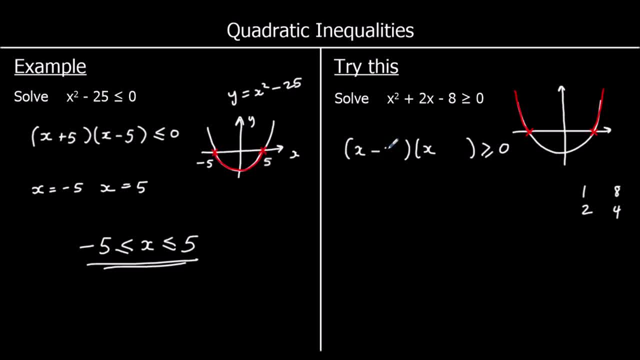 I make a positive 2 or I can have negative 2 and plus 4. so where does it cross the x-axis? so it crosses x at x equals 2. that makes the first bracket 0, and x equals negative 4 to make the second bracket 0. so we've got negative 4 and 2. we want the red parts of the graph. so what are the x? 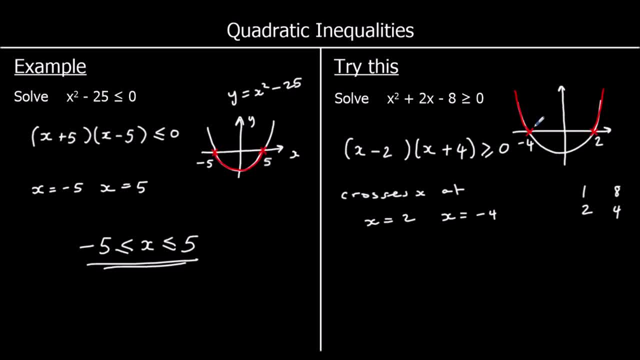 values in those parts of the graph. well, x is less than and it can equal, so less than or equal to negative 4. and the other one, x, is bigger than or equal to 2. so anything less than or equal to negative 4 or anything bigger than or equal to 2 will make this x squared plus 2x minus 8, bigger or equal. 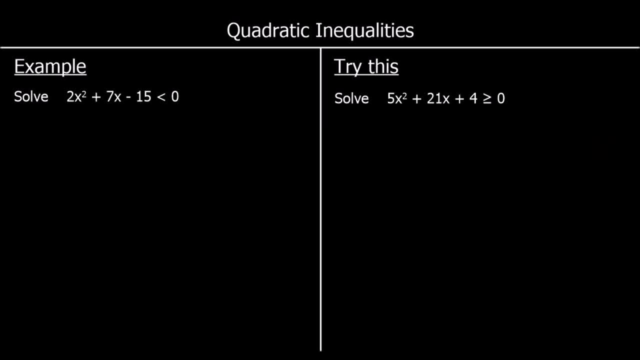 to 0. here we have another example. we still have a quadratic. we still want to find out what makes it less than 0 in this case. but the difference is we've got a number in front of the x squared, so quadratics are in the form. 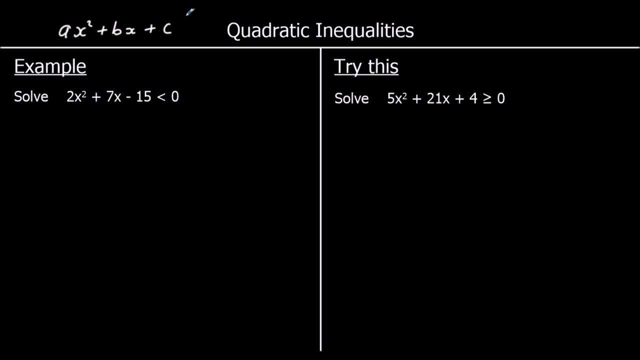 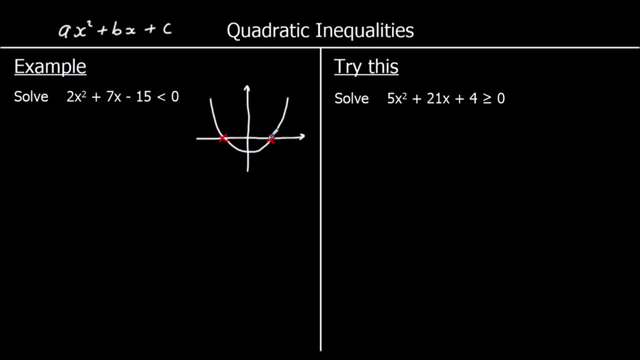 We can try factorizing it, and if it doesn't factorize, we can use the quadratic formula. So let's try and factorize it first. So I'm going to put 2x in one bracket and x in the other bracket, because 2x times x makes 2x squared. 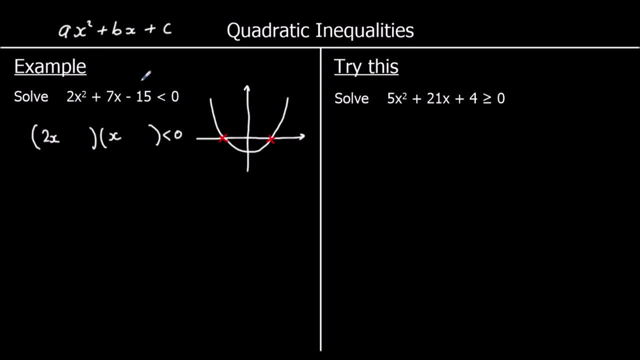 And then I'm going to do a times c. So I'm going to do 2 times 15 to get 30, and I'm going to look at what numbers multiply to make 30, and add to make 7.. But because I've doubled 15,, I've multiplied by 2, I'm going to divide one of them by 2 afterwards. 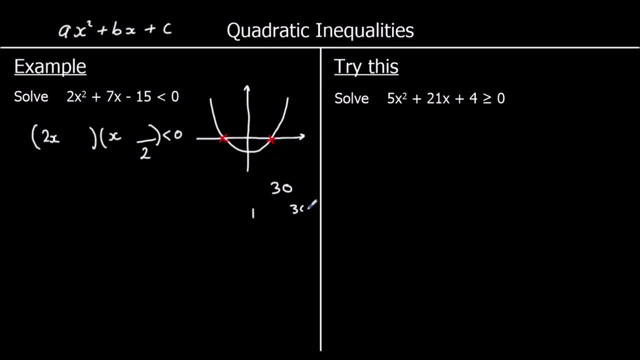 So what multiplies to make 30?? 1 30,, 2 15s, 3, 10s. It's not in the 4 times table And it's It's 5, 6s. So how can I get 7?? 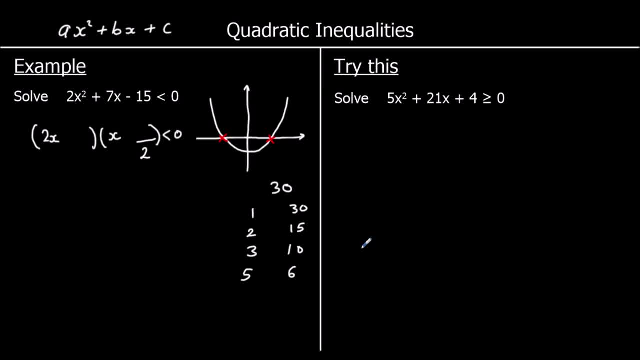 We can have negative 3 plus 10. So negative 3 plus 10. And I've put the 10 over 2, because that will simplify. So now we can find where it crosses the x-axis. So it crosses x. 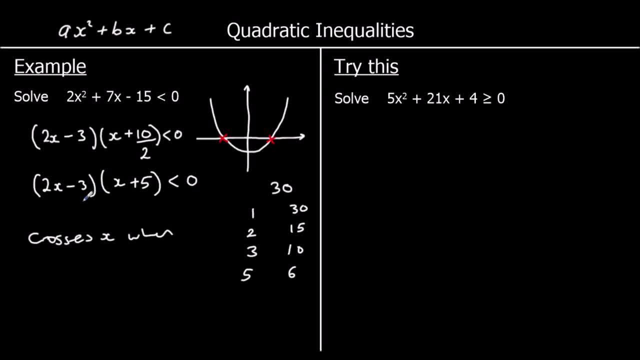 When? So what does x have to be for the first bracket to be equal to 0?? So if 2x minus 3 is equal to 0, plus 3 to both sides, So 2x is 3, and then divide both sides by 2.. 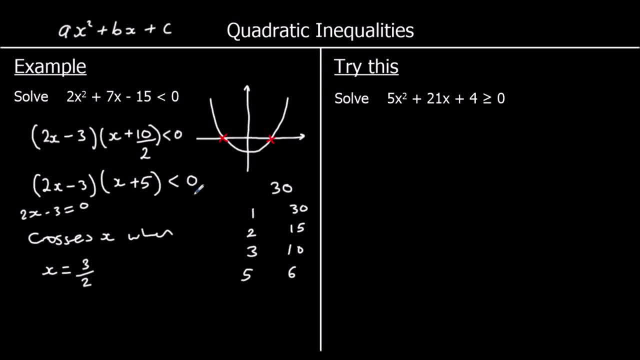 So that's 3 over 2, 1 and a half. And the second bracket: what does x have to be to make it 0? That's negative 5.. So we can say it crosses the x-axis at negative 5 and 3 over 2.. 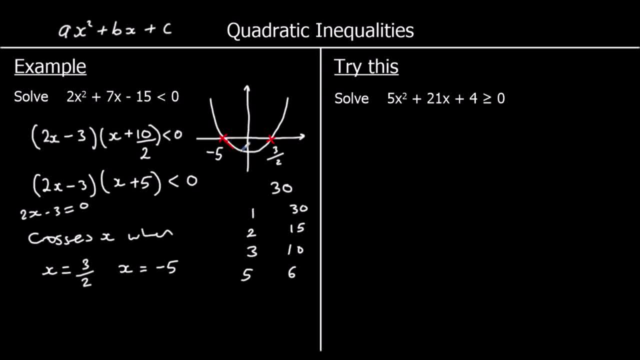 So what is, What are the x coordinates, the x values for this part of the graph where it's less than 0?? So it's bigger than negative 5 and less than 1 and a half, Less than 3 over 2.. 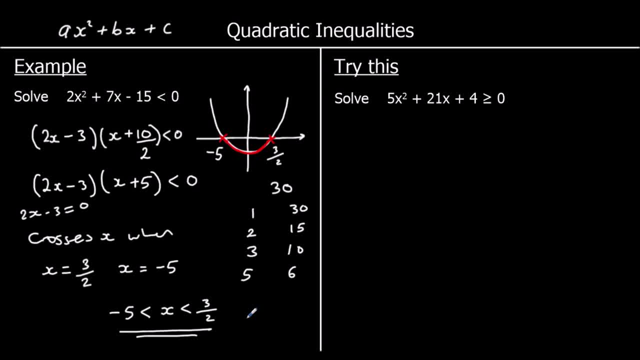 Okay, one for you to try, So give it a go. So we want where it's bigger or equal to 0 this time. So it's going to be bigger than 0 on these parts of the graph, So let's factorise it. 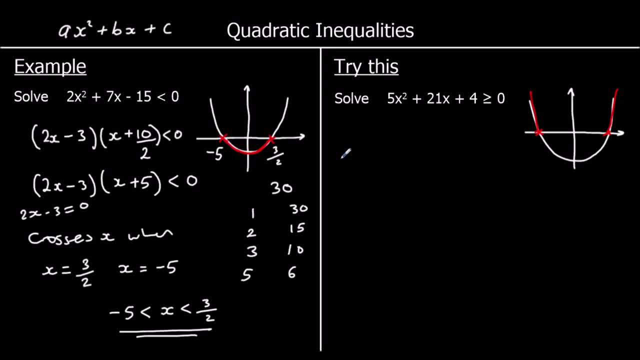 You can use the quadratic formula if you prefer, but I'm going to factorise here. So we've got 5x in one bracket, x in the other bracket. I'm going to do a times c, so 5 times 4, which is 20.. 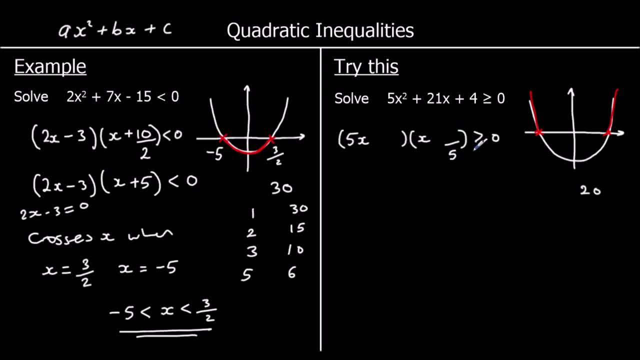 And because I multiply by 5, I'm going to divide by 5.. So divide one of the numbers I find by 5.. So we've got 1 times 20, 2 tens or 4 fives. How can I make a 21?? 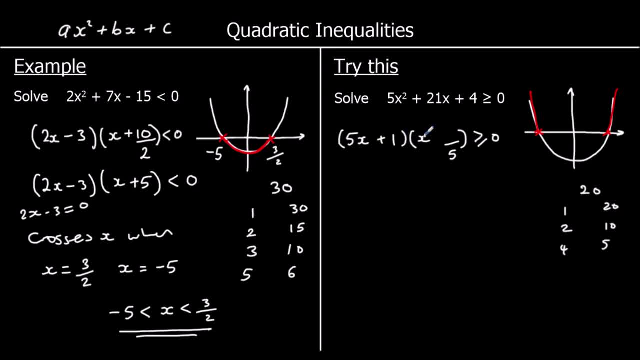 It's 1 and 20, and it's plus 1 plus 20.. So my graph doesn't look accurate, but that doesn't matter. So we've got 5x plus 1 and x plus 4.. So it crosses the x-axis. 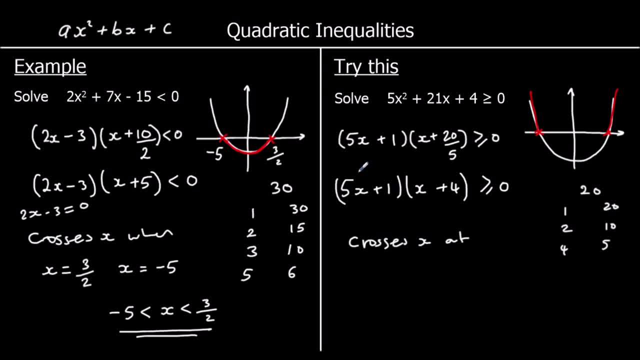 So it crosses x-axis. So what makes the first bracket 0?? That's going to be minus 1 fifth. And what makes the second bracket 0? That would be negative 4.. So it's negative 4 and minus 1 fifth. 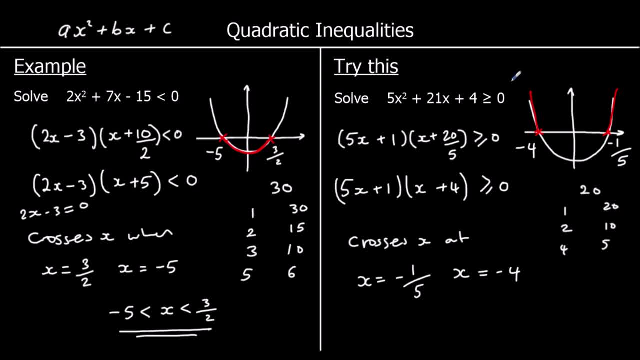 And we want the outside bits where it's above the x-axis, where it's greater than 0. So x is going to be less than negative 4 or greater than negative 1 fifth. So anything less than 4 or greater than negative 1 fifth will make this more than 0 or equal to. 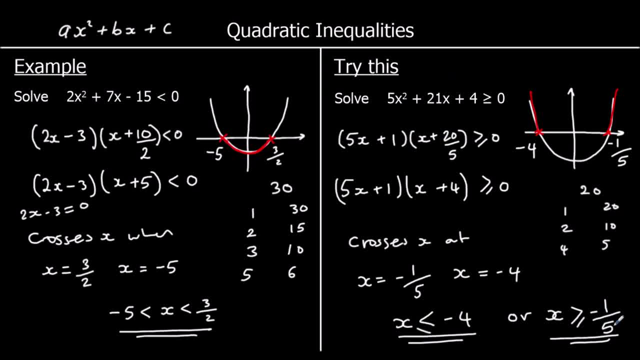 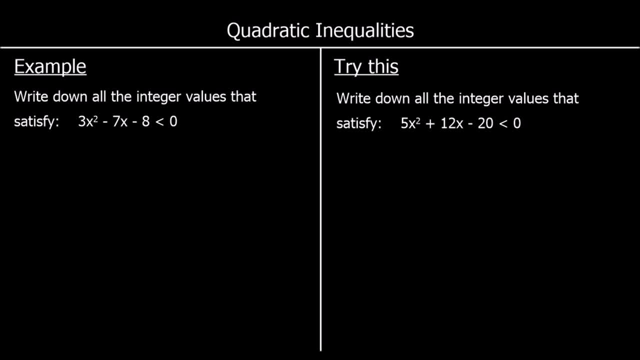 So it can equal negative 4 and it can equal minus a fifth. And one more example. This time the question says: write down all the integer values that satisfy 3x squared minus 7x minus 8 is less than 0.. 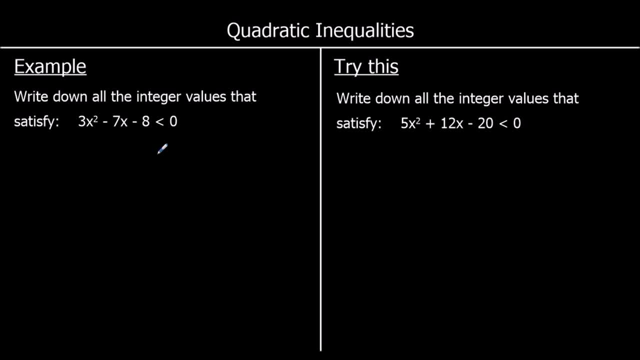 So we're only looking for the whole numbers that make 3x squared minus 7x minus 8, less than 0.. So again we've got a quadratic. So it's shaped like this: It's a positive x squared. 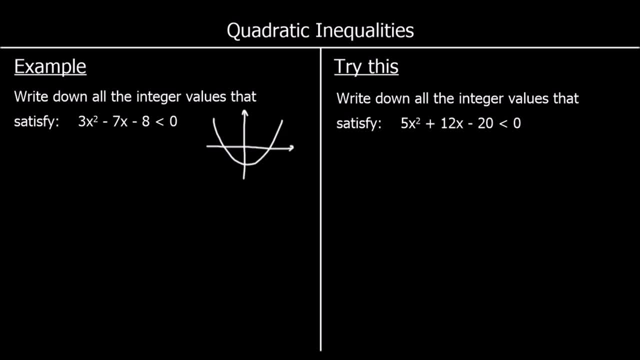 So it's a u-shaped graph, And we can find the points where it's equal to 0, where it crosses the x-axis, and use them to find out where it's less than 0. And then we can just give the answer as the whole numbers in between. 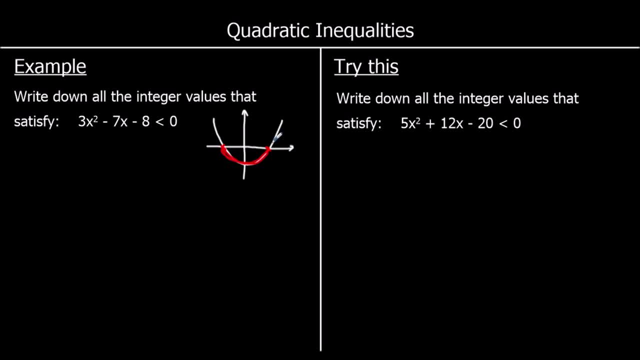 These two points, So whatever the whole numbers in between these two points are, will be our answer. So this time it won't factorize. but I only know that because I wrote the question So we can check. it doesn't factorize if we do a times c. 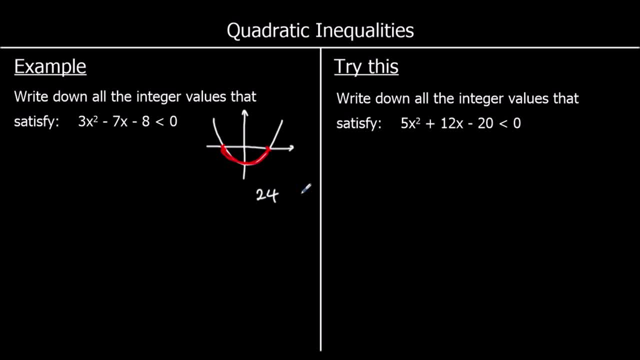 So 3 eighths, which is 24.. And write down the factors of 24.. And we'll see that none of them can make a 7.. So 124.. 2 12th, 3 eighths. 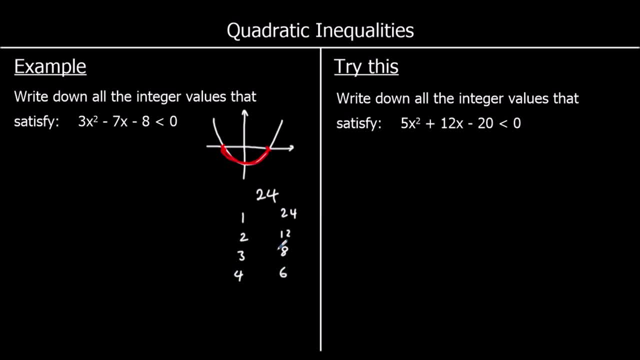 And 4 sixths. None of these options make a 7. So it won't factorize. We can't factorize it, So we're going to use the quadratic formula. So it's in the form ax squared plus bx plus c. 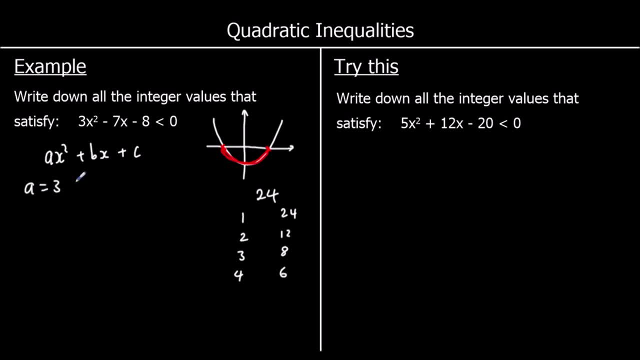 And so a is 3.. b is negative 7. And c is negative 8. And the quadratic formula says that x is equal to minus b, plus or minus the square root of b, squared minus 4ac, all over 2a. 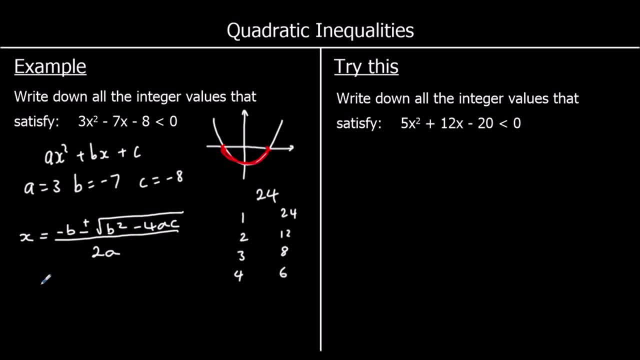 So we're substituting our a, b and c, which gives us minus, negative 7, plus or minus the square root of negative 7 squared minus, minus, 4 times 3 times negative 8, all over 2, 3s. 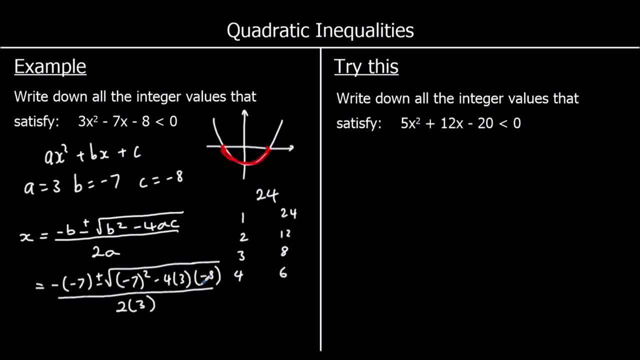 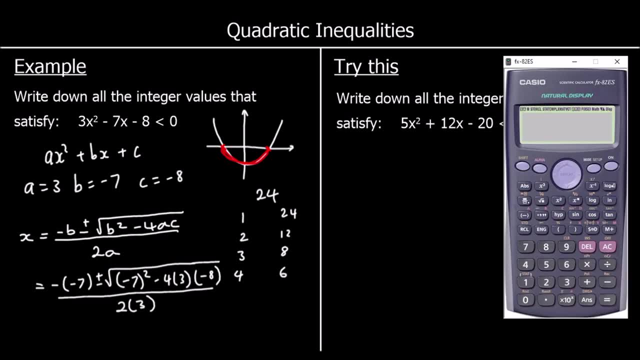 So let's grab a calculator and type it in. We'll have once with a plus and once with a minus to get two different answers. So negative minus, negative, 7.. I'll do plus first. The square root of negative 7 squared. 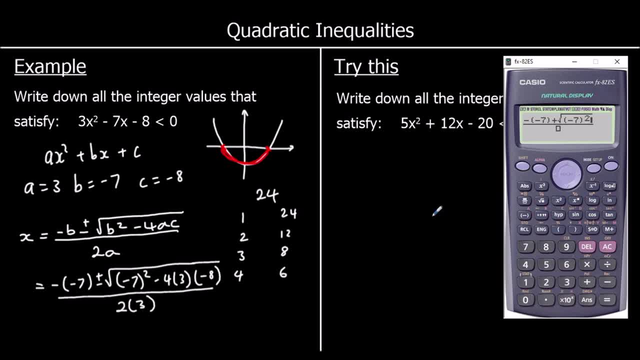 I'm putting my negative 7 in brackets, Otherwise the calculator wouldn't do it correctly. Minus 4 times 3 times negative 8, all over 2, 3s. So I've got 3 point. I'll just write down 3.2 to one decimal place. 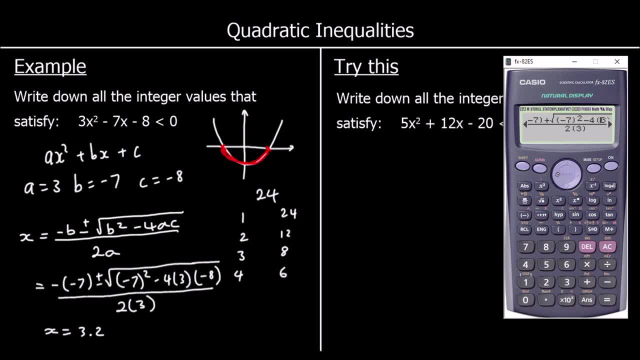 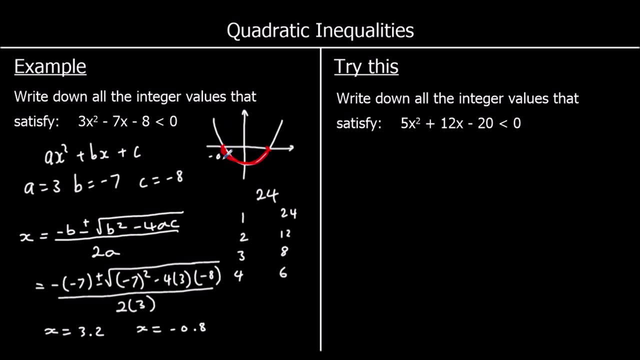 And I'm going to click back in to change So plus to a minus And that will give us our second answer of minus 0.8.. So we've got negative 0.8 here. We've got 3.2 here. 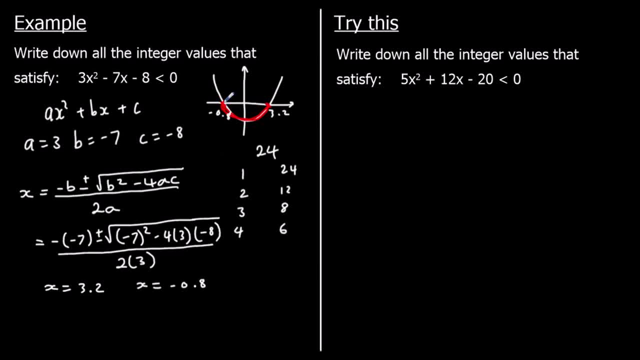 So what are the whole numbers in between them? So that's 0,, 1,, 2, and 3.. So 0,, 1,, 2, and 3 are the only whole numbers that you can substitute in here to make it worth less than 0. 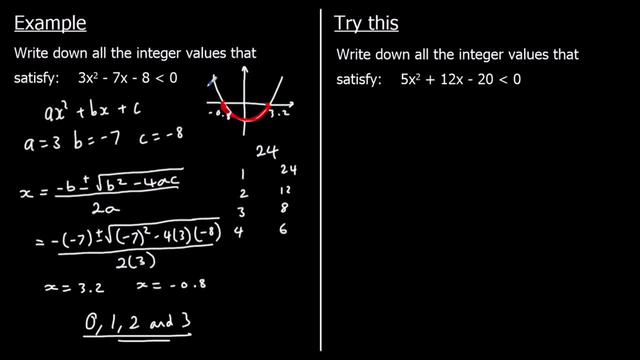 Okay, one for you to try. So the same sort of thing, Give it a go. So again, we're going to use the quadratic formula. We've got a is 5.. We've got a is 5.. B is 12.. 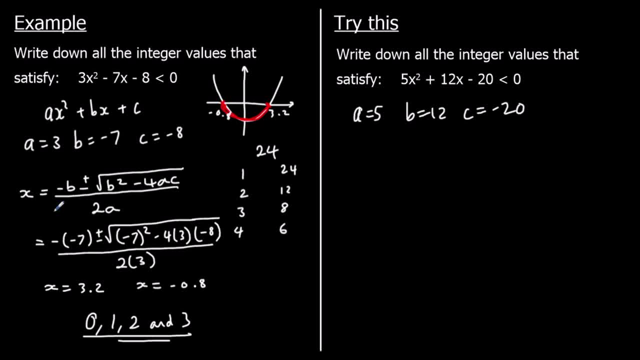 And C is negative 20.. So the quadratic formula is written down here And we're going to substitute in our A, B and our C. So we're going to have minus 12, plus or minus the square root of 12, squared minus 4 times, 5 times negative 20.. 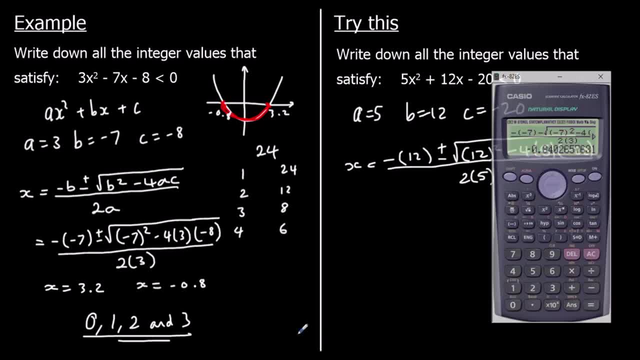 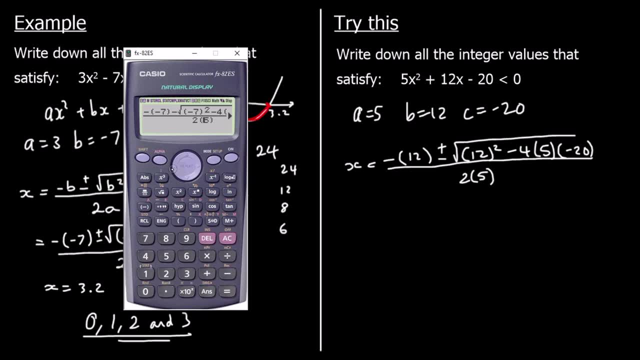 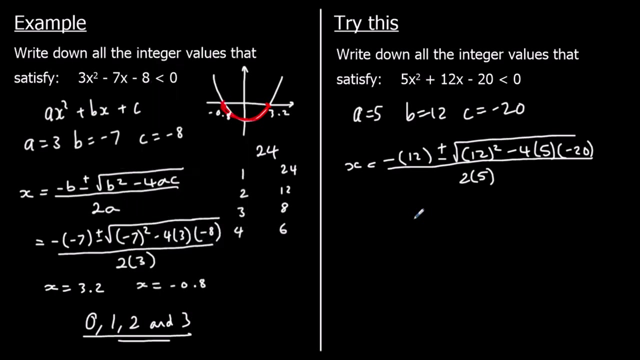 All over 2, 5s. Let's type it in the calculator Once for a plus and once for a minus. We'll do the plus first. So we've got 1.1., 1.. And if we change the plus to a minus? 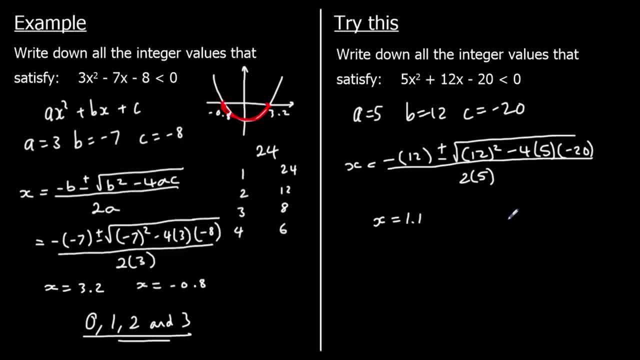 We get negative 3.5.. So we want, We want The values that make it less than 0. So we've got negative 3.5 and 1.1.. And we want the whole numbers in between them. 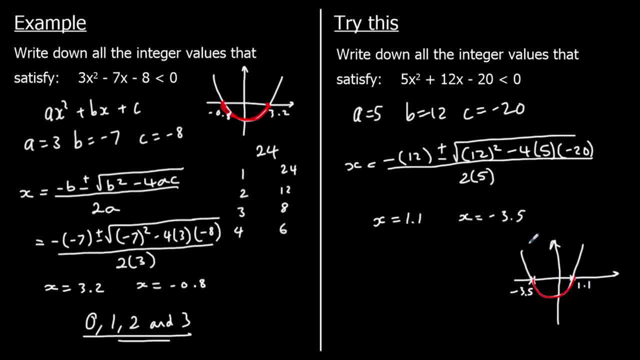 So the whole numbers in between negative 3.5 and 1.1.. Which is negative 3, negative 2, negative 1, 0, and 1.. So negative 3, negative 2, negative 1, 0, and 1.. 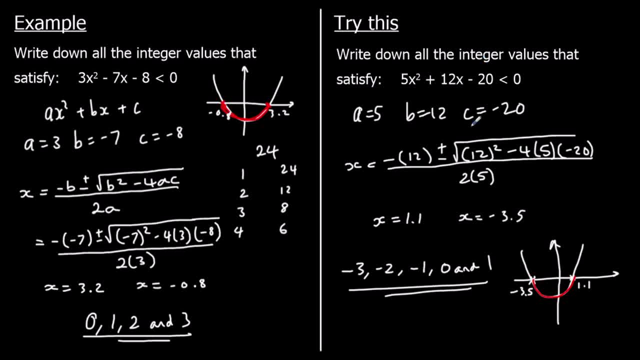 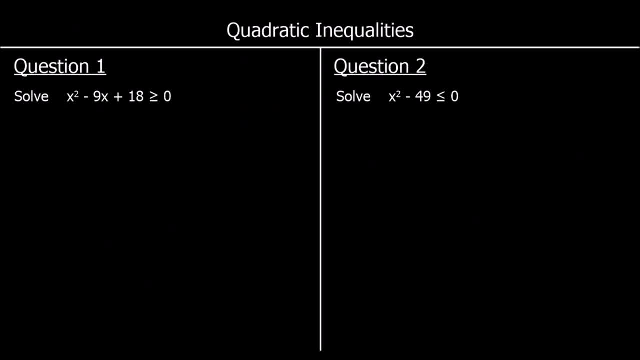 If we substitute them in here, it will be worth less than 0.. Okay, let's finish up. Two questions. Pause the video, Give them a go And press play when you're ready for the answers. Question 1. Solve x squared minus 9x plus 18.. 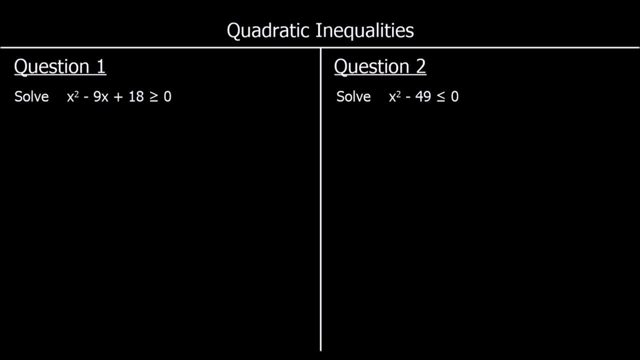 Is bigger or equal to 0. So it's going to look So you don't have to. If you're going to do a sketch, you don't have to do it accurately, It doesn't matter if you get it completely wrong. 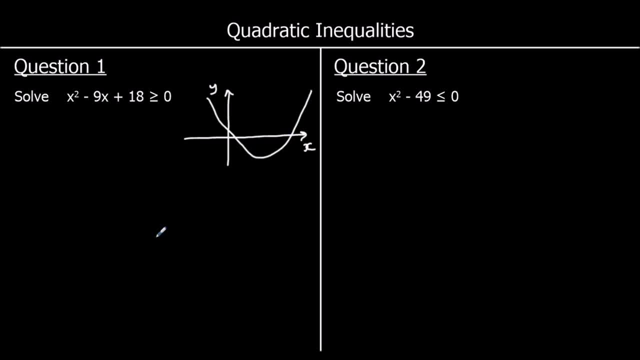 It's just for your To help you with the working out. So it's going to look something like this, And We want where it's bigger or equal to 0.. So if we find what makes it equal to 0.. 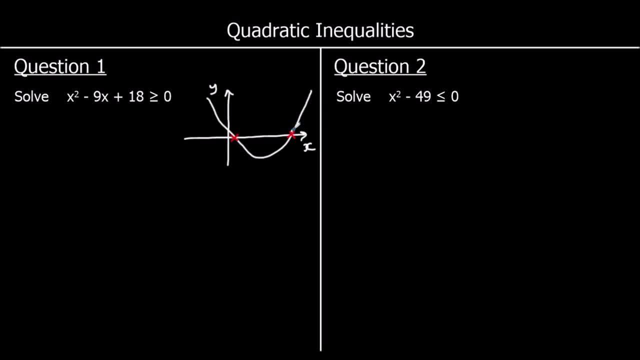 That would be Where it crosses the x-axis And it's bigger than 0 above the x-axis. So we're looking for these parts of the graph Up here. So let's solve it, And we'll do that by factorizing. 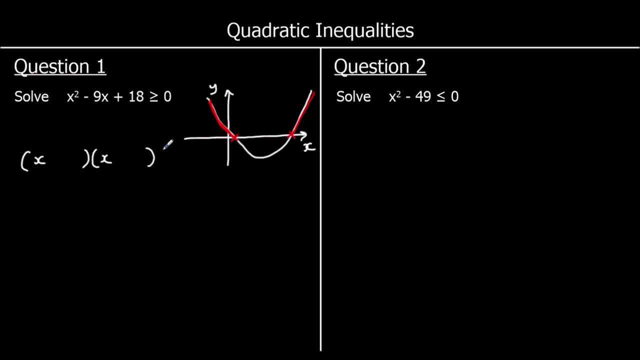 So we're going to have x in both brackets. x times x makes x squared. What multiplies to make 18? 1, 18.. 2, 9s And 3, 6s. Which of those can give me a negative 9?? 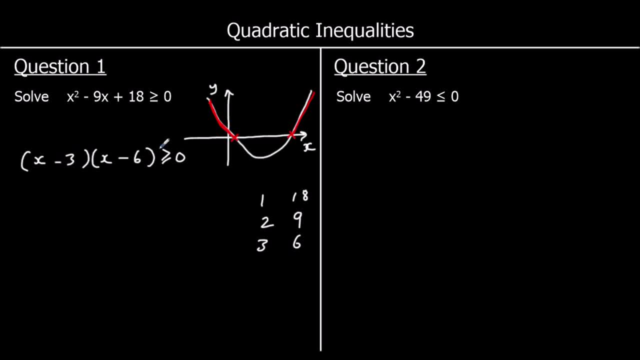 Negative 3 and negative 6.. So it crosses x At x equals 3.. That makes the first bracket 0. And x equals 6. That makes the second bracket 0. So where is it bigger or equal to 0?? 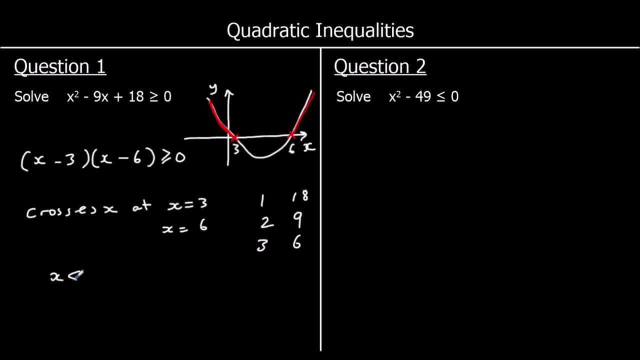 So it's where it's less than Or equal to 3.. Or where it's bigger or equal to 6.. Question 2. Solve x squared minus 49 is less than or equal to 0.. So again we've got a quadratic graph.